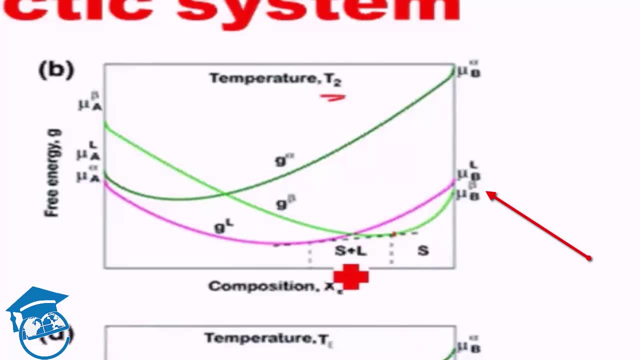 Till here, beta is the lowest energy phase. From here till here, the tangent has the lowest energy phase. Therefore we will have beta plus liquid, and over here, over the remaining region, liquid is still now the lowest energy phase. So let's see temperature: T2 till here. 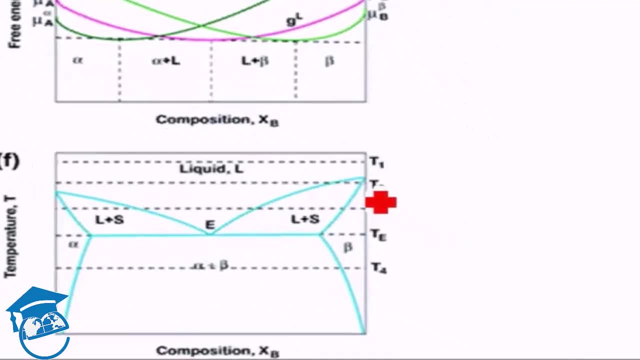 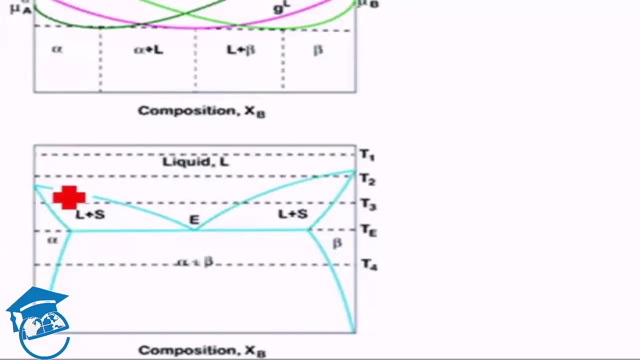 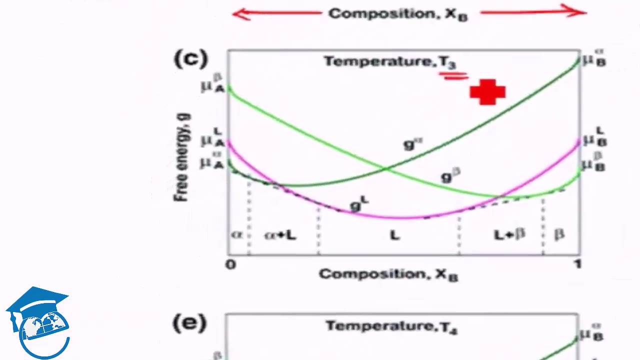 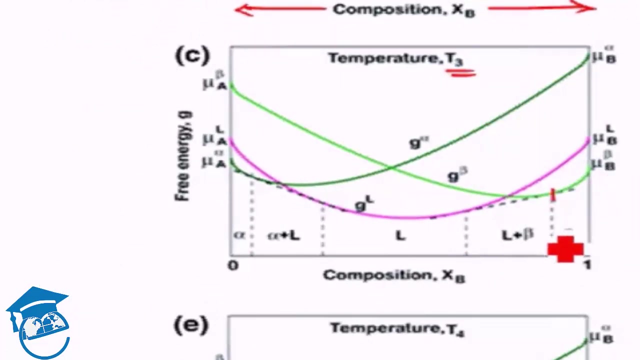 we have solid beta, We have beta, Then we have liquid, solid liquid plus beta. Then we have the liquid Right. Next we take temperature T3. In temperature T3 what is happening is beta is of the lowest free energy for certain region. Then we have liquid plus beta because 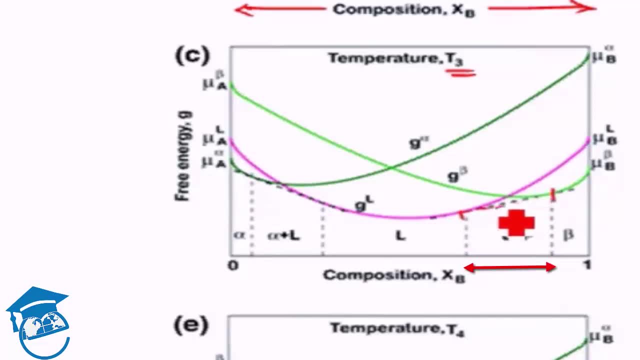 the combination has lower free energy than any individual phase. Then we have some region which has the liquid as the minimum free energy phase, But we also have got here alpha, which is the minimum free energy for certain region, and then alpha plus liquid. Okay, We got alpha. 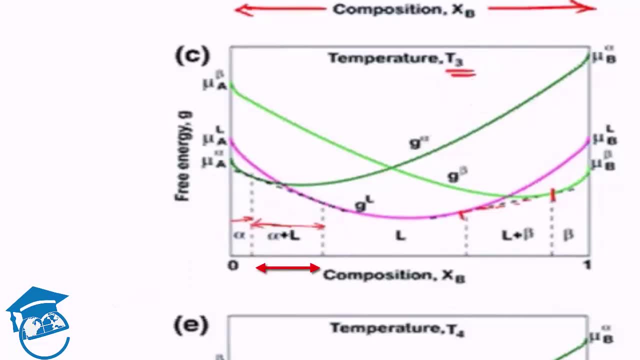 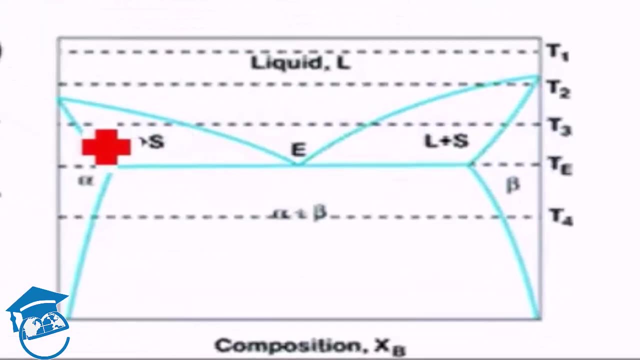 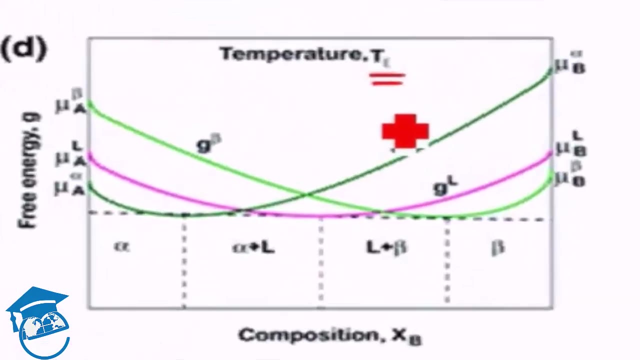 plus liquid. Let's replicate it here: T3. We come T3. So beta, beta plus liquid. So beta plus liquid liquid, alpha plus liquid alpha. Now let's go to eutectic temperature: Te. At eutectic temperature there has to be invariant point, That is a point where three phases 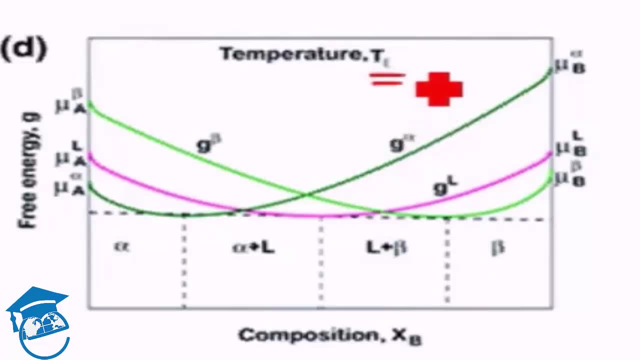 will coexist. I forgot to mention this, But at this eutectic temperature, eutectic composition, we have three phases coexisting. Let's see Beta stable liquid plus beta stable, liquid stable, alpha plus liquid stable, alpha stable. And this point, at exactly this point all. 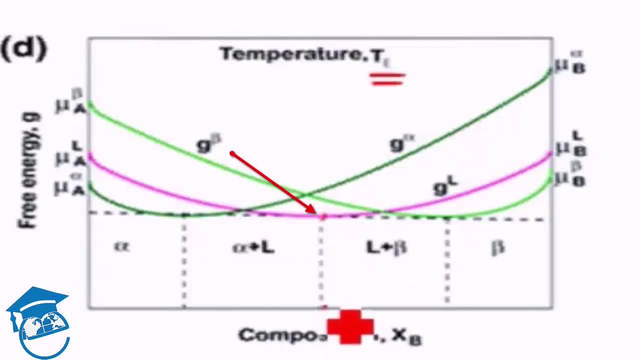 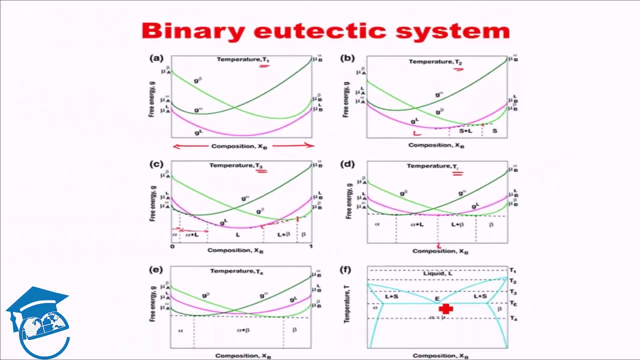 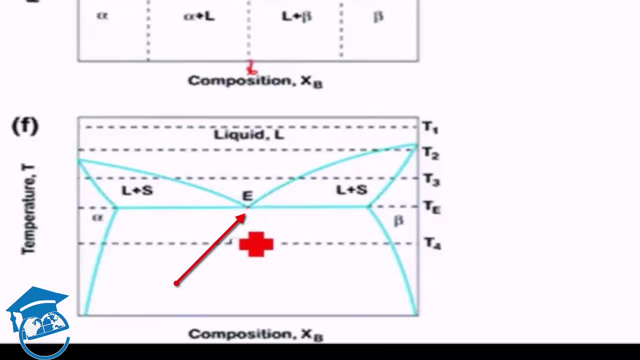 the three alpha plus liquid plus beta is stable. It's just a singular point. Let's draw it here: Beta, beta plus liquid. alpha, alpha plus liquid. Meeting point: liquid plus alpha plus beta. Finally, at any temperature below the eutectic. 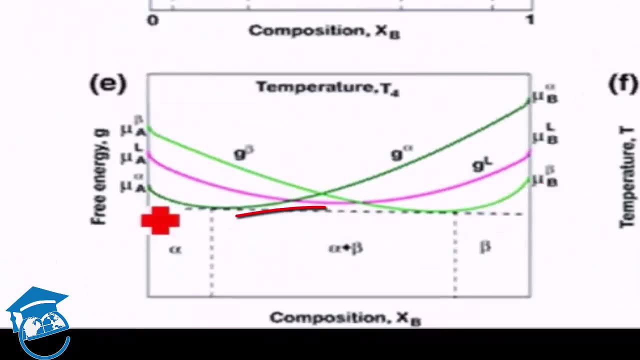 temperature we will have stable beta, stable alpha and stable alpha plus beta. Nowhere does liquid have minimum free energy. Independently or in combination, Liquid does not have free energy which is minimum at this temperature. Let's plot that: T4.. Beta alpha, alpha plus. 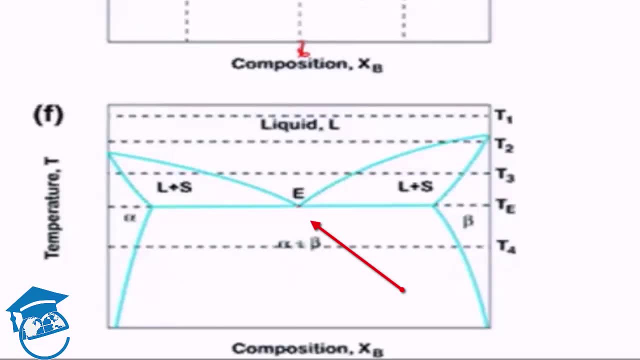 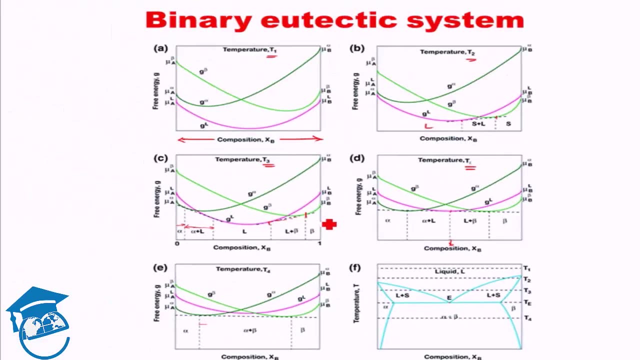 beta. Okay, So using different temperatures- free energy temperatures- we found out which phase is stable, for what composition range. We plotted that and, combining all the temperature information, we got the phase diagram for a eutectic system. Just to round it up, this is the invariant point, which has zero degree of freedom and 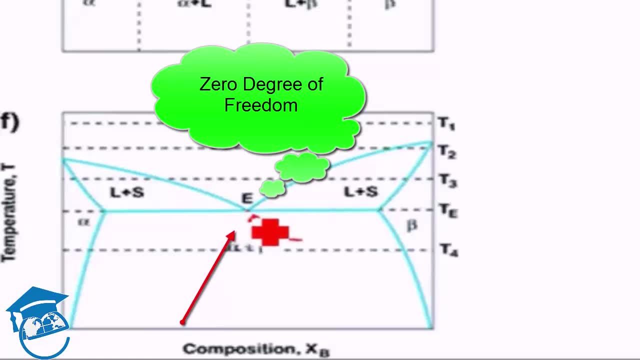 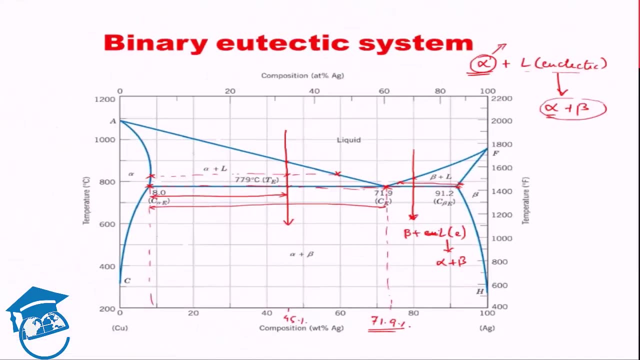 where three phases coexist. Okay, One important thing is that in a phase diagram if you draw a isothermal line anywhere in the phase diagram, a isothermal line, you will always attain alternating regions of single phase and double phase. for a binary phase diagram: Single phase, alpha, double. 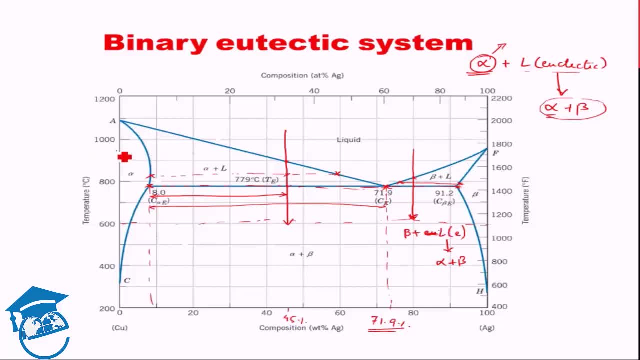 phase: alpha plus beta. single phase alpha. Try to draw it here. What do you get? Alpha- single phase. double phase. single phase liquid. double phase, liquid plus beta. single phase beta. It will always happen. If this is not happening, you have. 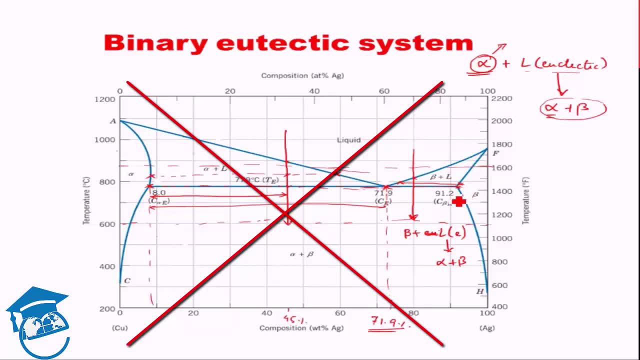 not drawn the phase diagram correctly. Okay, So this is, I guess, more than enough for you eutectic systems. We might revisit this when we discuss about iron carbon phase diagram. Or at least, if you are interested, please refer to the video on iron carbon phase diagram. 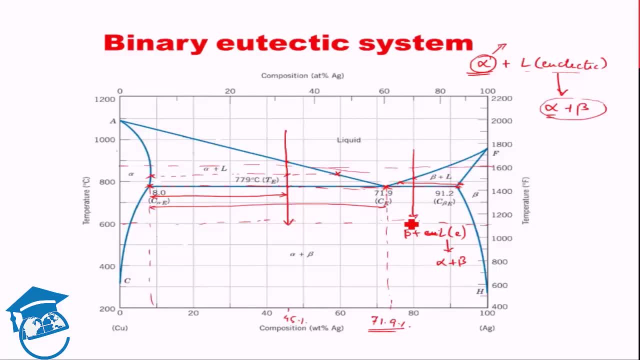 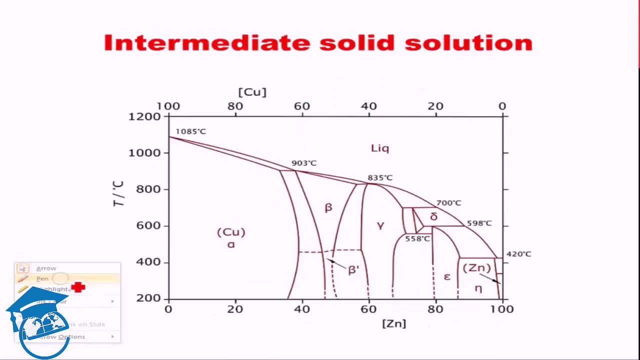 we will see the eutectic reaction taking place in iron carbon phase diagram later. Now, apart from isomorphous system and eutectic system, we have other systems also which has intermediate solid solutions. In the eutectic system, what we saw? we had terminal solid solutions. 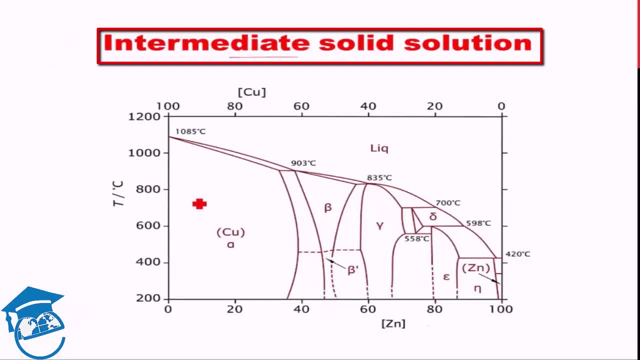 There was alpha at one end, beta at other end, But there can be systems like zinc copper system. This is zinc copper system which has intermediate. This is the terminal solid solution, alpha, and over here there is another terminal solid solution. But in addition to them, you 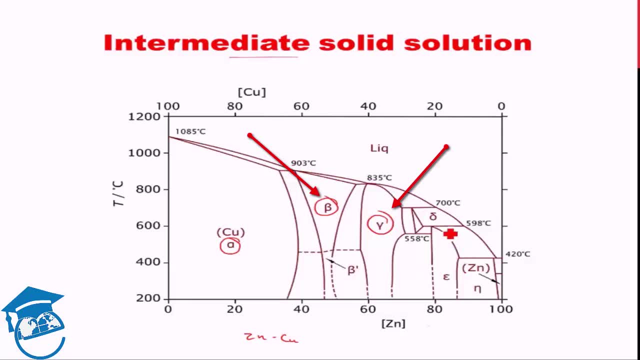 have beta, you have gamma delta, So there are multiple solid solutions which can be used which do not lie at the edge Right. So these are called intermediate solid solutions And this type of diagram might look quite complicated, but the basic fundamentals, how? 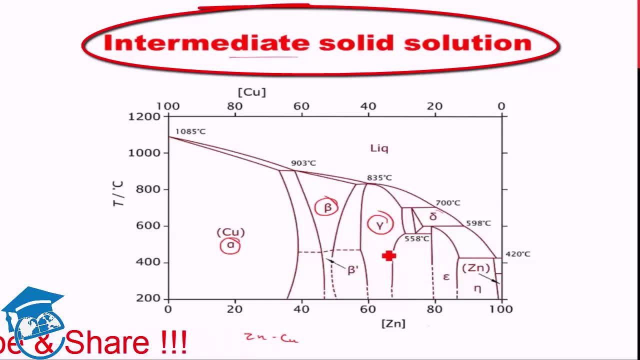 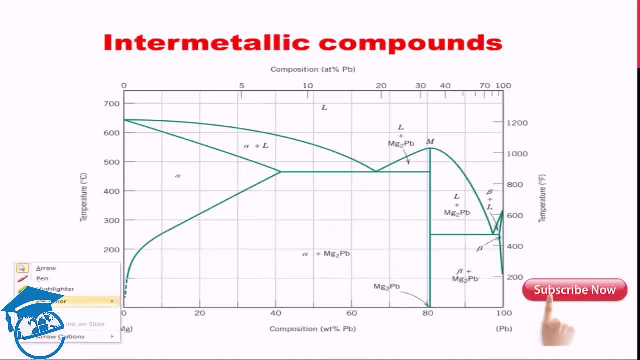 they are made and how information can be extracted from this are the same. Then we again have something which is known as the intermetallic compound. Ok, Till now, what we have seen is any phase which existed in a phase diagram was a region like. 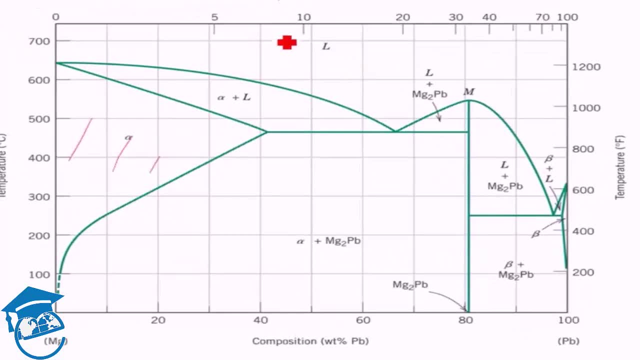 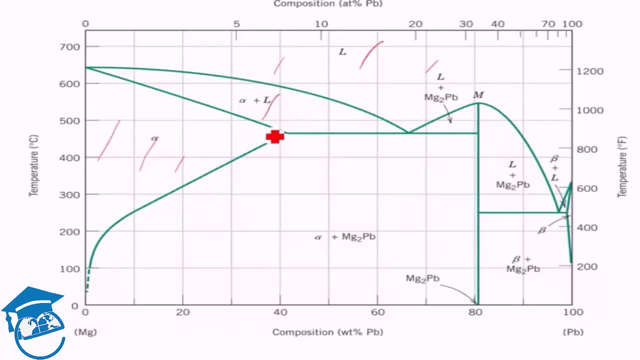 it was either a region alpha or a region liquid. We had alpha plus liquid region, But it can so happen that instead of a region it forms a line compound, That is, it forms a compound which does not lie in a region, but it is a singular line. 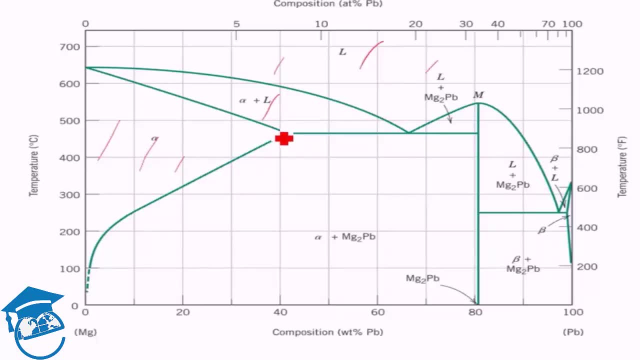 It is only at a specific composition rather than a range of composition. Here it is This: at around 81%, what we have is Mg2Pb in magnesium lead phase diagram. This is a singular line, Right. It is not an area, It has a fixed composition And this type of compounds which are formed 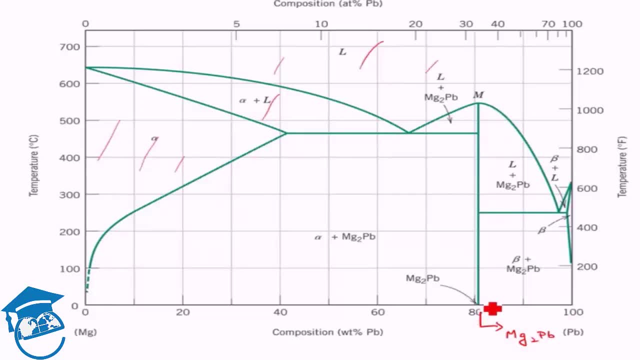 in a phase diagram, which do not occupy an area, are known as intermetallic compounds. So a point to take home here is that this is considered as a single phase region, though it is a single phase line. Why do I say this? I say this because when you try to see the